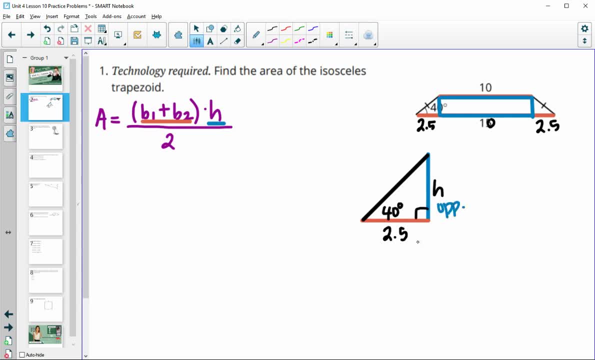 got the 40 degree angle. So this is the opposite side and this is the adjacent side. So we're going to be doing a tangent function. So we're going to be doing: tangent of 40 equals the opposite side, H over the adjacent side, 2.5.. And then we'll multiply that 2.5 up. So we're doing 2.5. 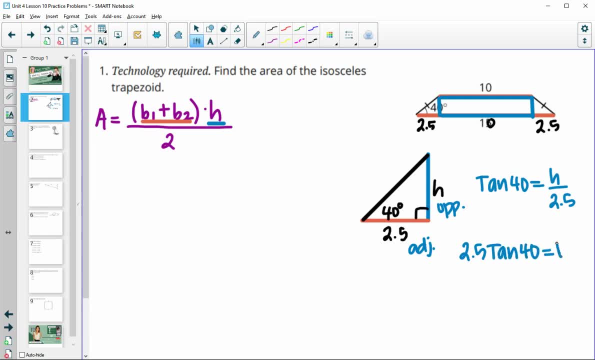 times the tangent of 40 in our calculator And that will give us a height of 2.1.. So now we know kind of all of the things for this formula. So we're going to add these bases together, multiply by the height and then divide by 2.. So our bases were 10 and 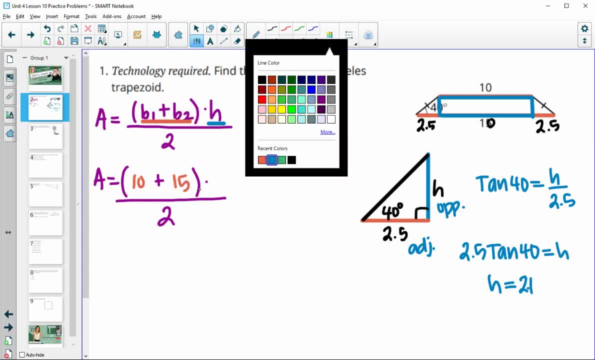 15.. And then the height that we just solved for was 2.1.. So we'll type that into our calculator and we'll do 25 times 2.1, which is 52.5 divided by 2., And that gives us an area of 26.25 units. 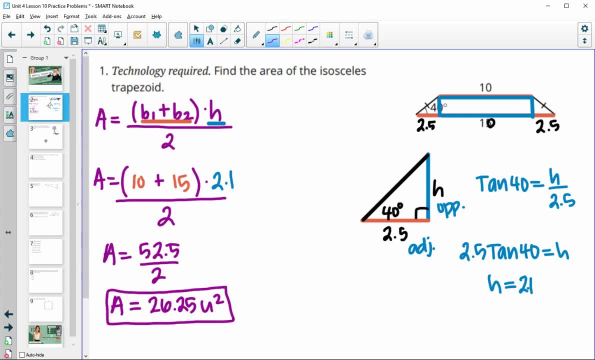 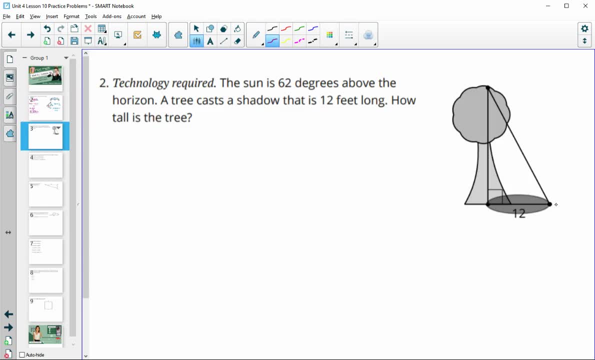 squared. Number two: the sun is 62 degrees above the horizon, So that would be this angle going up here in this diagram, And it creates a 12 foot long shadow. How tall is this tree? So when we take a look here? so we've got this angle- the height is the opposite side. 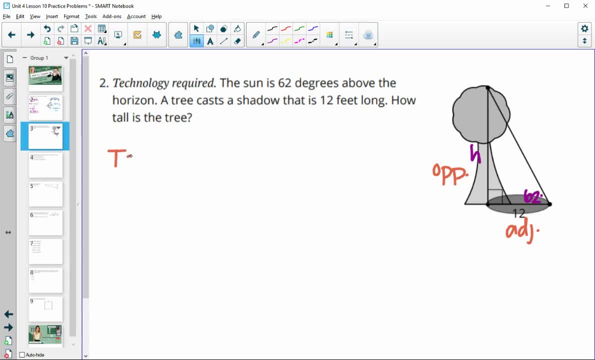 The shadow is the opposite side. So we're going to take a look here. So we've got this angle: the height is the opposite side And then the height is the adjacent side. So we again have a tangent function, So tangent of 62. 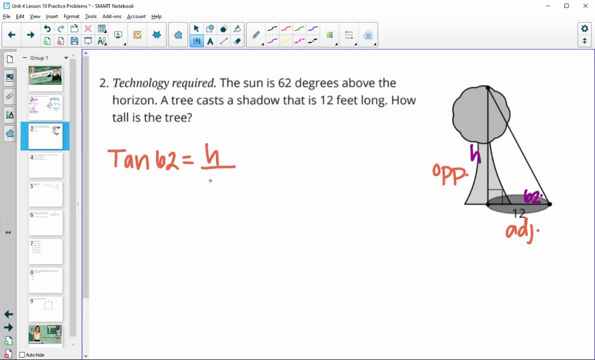 equals the opposite side h over the adjacent side 12.. And then we can multiply this 12 up, So we get 12 times the tangent of 62 that we can type in our calculator, And so 12 times the tangent of 62. 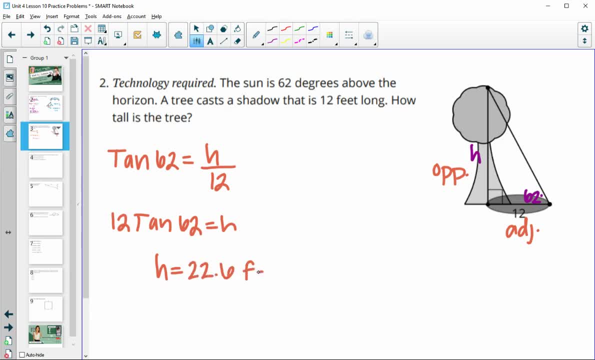 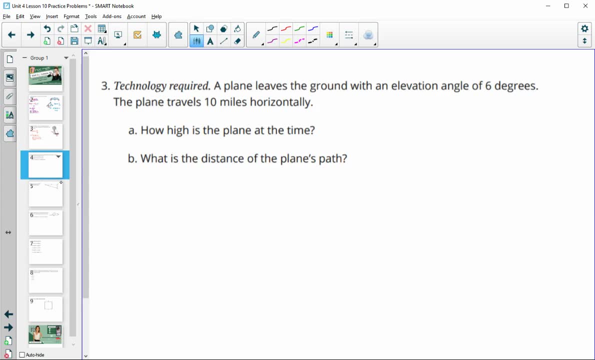 gives us 22.6. feet for the height of the tree. Number three: a plane leaves the ground at an elevation of six degrees. The plane travels 10 miles horizontally. Let's answer these questions. So we've got the ground here. Let me do it: green like grass. Okay, so we've got the ground here. 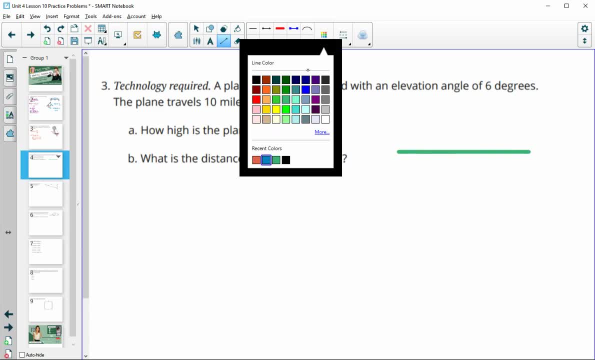 and then there's the elevation that the plane is traveling at a six degree angle, and then we want to figure out a couple different things here. So we've got this height that we're looking for, and then we're also going to actually be looking for this blue path. So we know that. 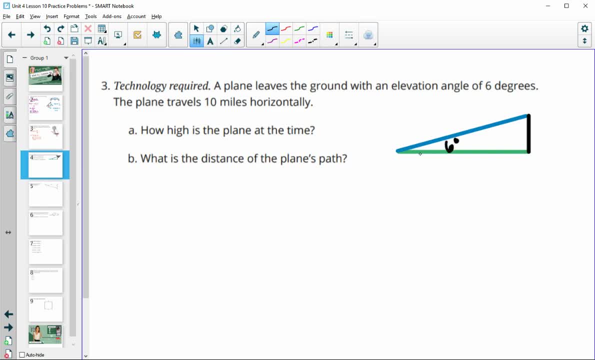 this angle here. they told us was six degrees and we know that the path, the horizontal path, they told us was six degrees. So we're going to be looking for this blue path. traveled is 10 miles, so the first thing that they're asking is: how high is the? 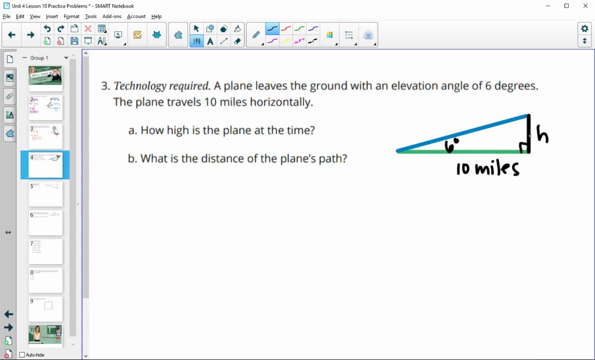 plane. so that's this segment here for the height above the ground, so this altitude. so if we go ahead and solve for that, from this 6 degree angle, the height is the opposite side and this horizontal distance is the adjacent side, so we'll be able to do a tangent function. so tangent of 6 equals the opposite side, H. 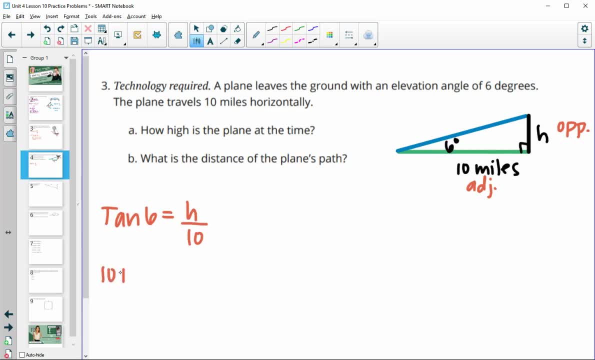 over the adjacent side 10. so we'll multiply that 10 up and we'll get 10 times. the tangent of 6 will give us our height. so the height in this case is going to be 1.05 miles. then it wants us to find the distance that the plane is. 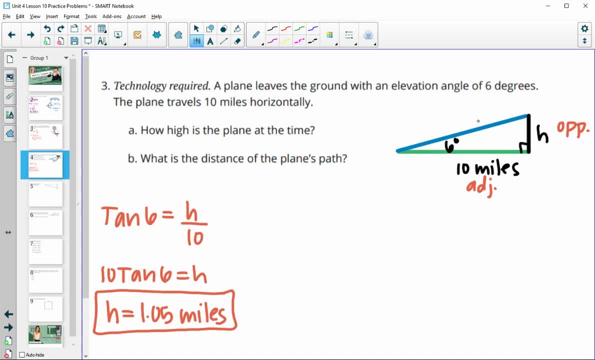 actually flying at and that's going to be the distance that the plane is actually flying at and that's going to be the distance that the plane is actually traveled. so the plane is flying along this blue line, so this is gonna be the distance actually traveled, and we know that that is the hypotenuse of the 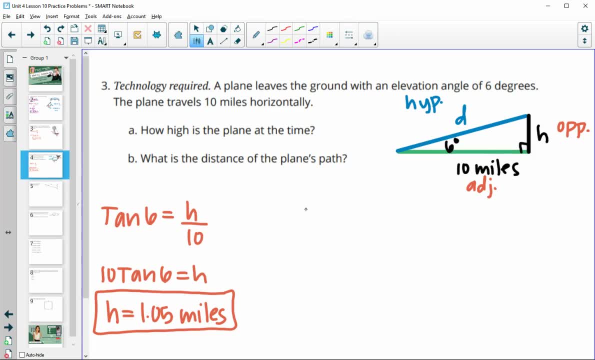 triangle. so you could use the 10 and the 1.05 in the Pythagorean theorem if you would like to. I'm just gonna set up a cosine function. so cosine of 6 equals the adjacent side 10 over the hypotenuse D, multiply the D up. 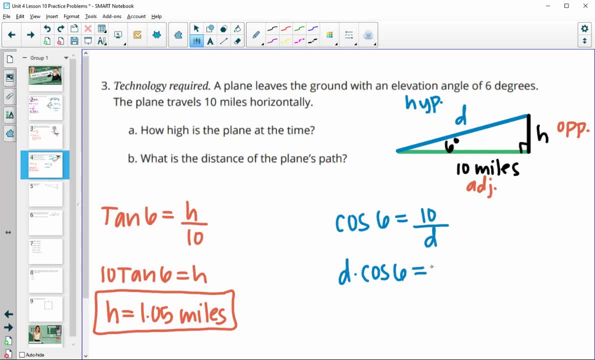 so 10 times cosine of 6 equals 10, and then we'll divide that cosine to both sides. so we're going to be doing 10 divided by cosine of 6 and that gives us an answer of 10.06 miles. when we type this into our calculator, number 4: find the missing. 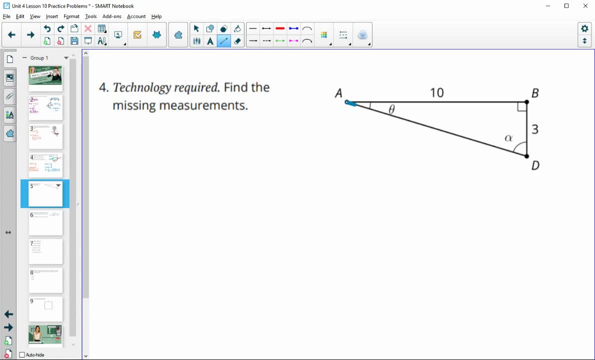 measures. so we need to find side A, D, so the hypotenuse, and then we're also going to have to find theta and alpha, the two angles. so let's go ahead and find this hypotenuse first. we know that we've got the other two side lengths, so 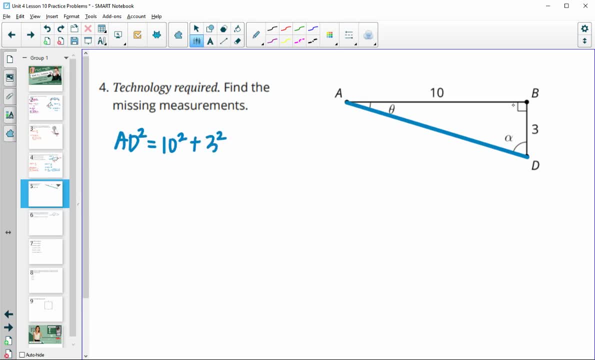 we're able to do Pythagorean theorem, since we see that it's also a right triangle. so a D squared equals ten squared plus three squared. so we're just gonna combine. So AD squared is equal to 100 plus 9, so 109.. 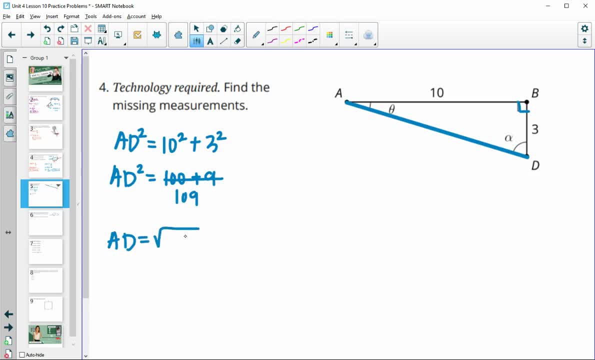 And then we'll square root both sides and we get the square root of 109 for that segment. You could also type that in your calculator and get a decimal of 10.4.. Then we just need to find the angle measures. So if we go ahead and find theta first, 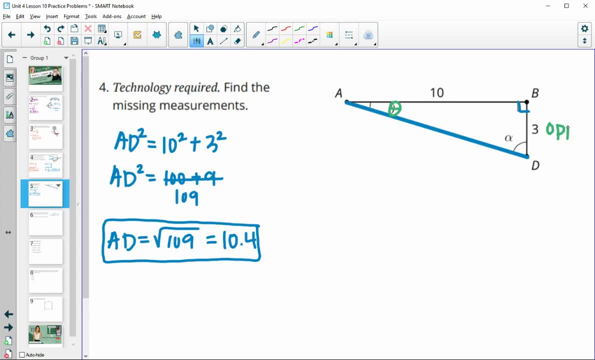 So I'm going to label this 3, the opposite side, since it's directly across from theta, And then the 10, the adjacent side. So I'm going to do an arctan function, So arctan of 3, the opposite, over 10, the adjacent. 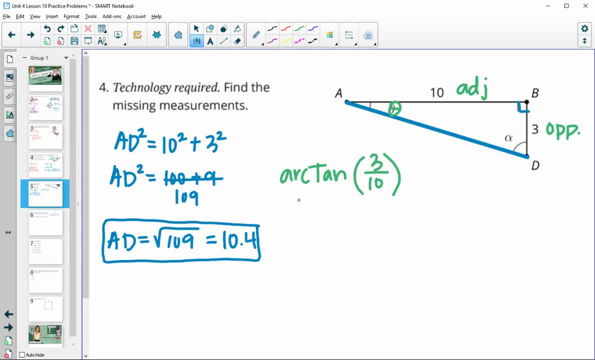 And then remember that arctan is also in your calculator as tan negative 1.. And so we'll type in the tan negative 1 of 3 over 10. And that gives us that theta equals about 17 degrees. Then to find alpha, remember that these two angles total 90, since we've already used 90 up. 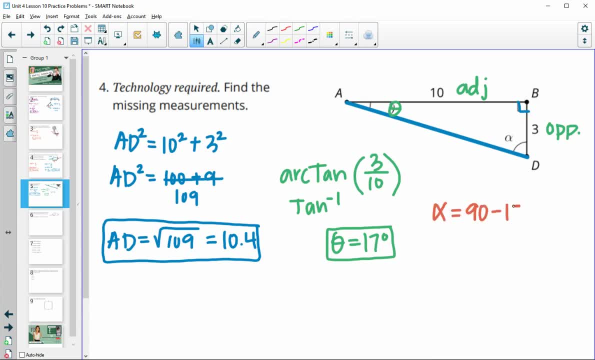 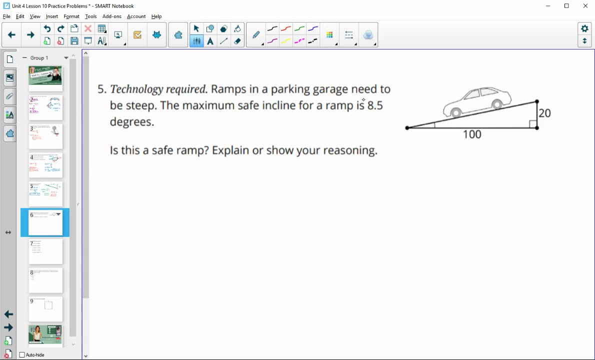 So alpha is going to equal 90 minus theta, So 90 minus 17.. So alpha is equal to 73 degrees. Number five: in parking garages the ramps need to be steep, but they have a maximum safe incline of 8.5 degrees. 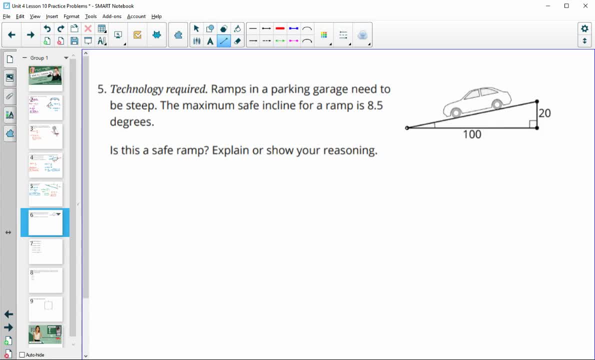 So let's decide if this angle here is too steep or if it's safe. So when we're looking at this angle, we need to label the sides. So across from this angle, since we're in a right triangle, across from this angle we need to label the sides. 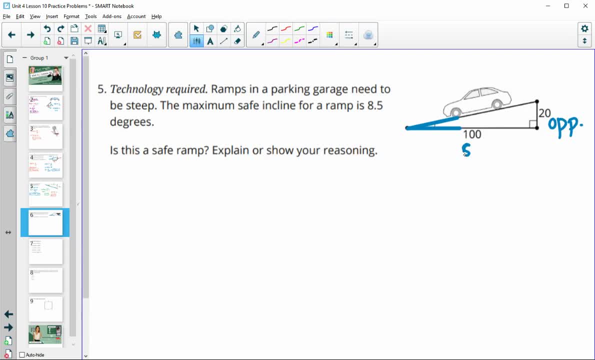 So across from this angle is the opposite side and next to it is the adjacent side. So in order to figure out this angle, we would do an arctan, since we have opposite and adjacent of 20 divided by 100.. And when we do that, remember tan negative 1 in your calculator. 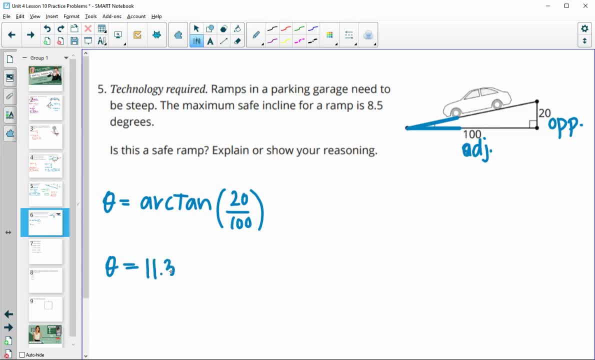 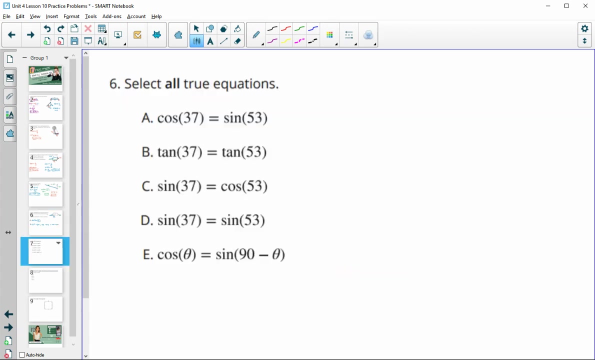 we get an angle measure of 11.3 degrees, which is not less than our 8.5.. So then, this is not safe. So, since this is greater than 8.5 degrees, the ramp is not safe. Number six: select all true equations. 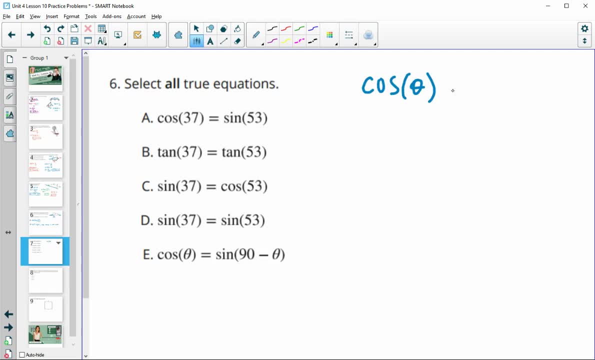 So remember that when we have a cosine of an angle, that that equals the sine of 90 minus that angle, Because when they're in the same triangle the sine and cosine of opposite angles are equal to each other. So we're good with A, because 37 plus 53 equals 90 and we've got a sine and a cosine. 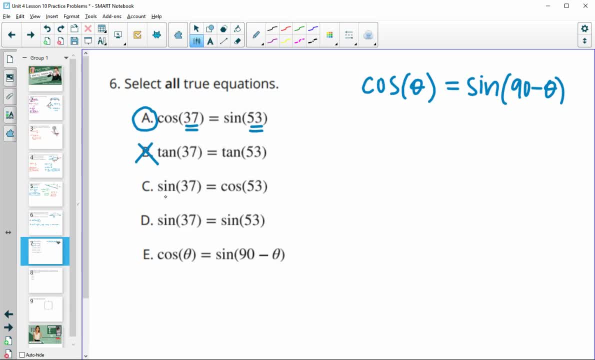 This does not hold true for tangent. So now in C we've got a sine of 37 and a cosine of 53. Those add to 90 and we've got a sine and a cosine, So that one's good D has both sine. 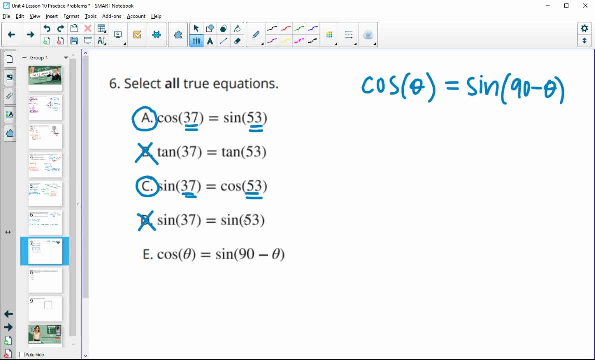 So that's not going to be equal, unless these numbers are equal. And then E is exactly the formula that I wrote. So these two angles, theta and 90 minus theta, would add to 90 and there's a sine and a cosine. So that one's good as well. 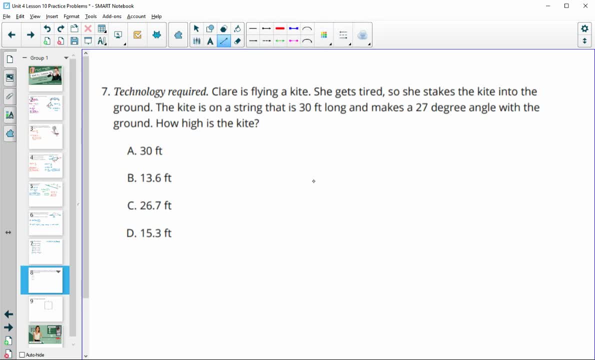 Number seven, Claire is flying a kite. She gets tired so she stakes the kite to the ground. The string of the kite is 30 feet and makes a 20. 27 degree angle with the ground. Let's figure out how high this kite is.